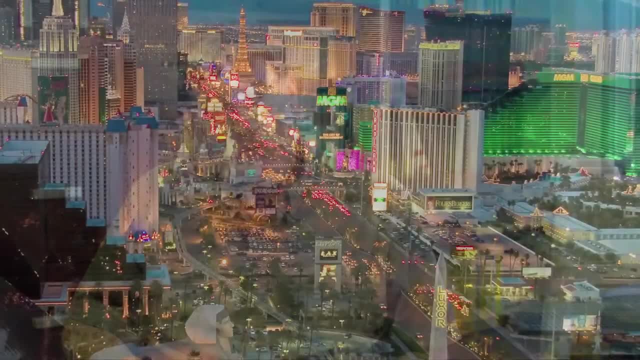 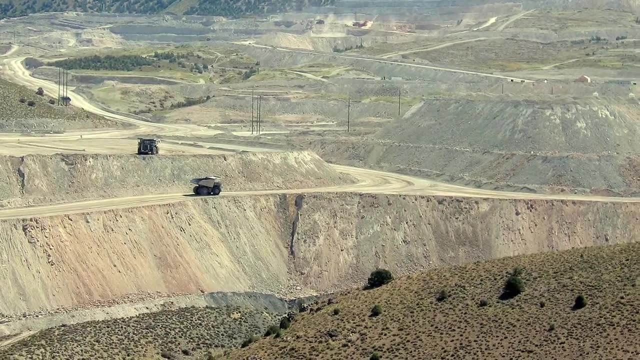 wide agency. So we do work in all corners of the state, including, if you will, the burgeoning city of Las Vegas, in the south, the major gold deposits in northeast Nevada and then in western Nevada, analyzing the earthquake potential and geothermal resources. 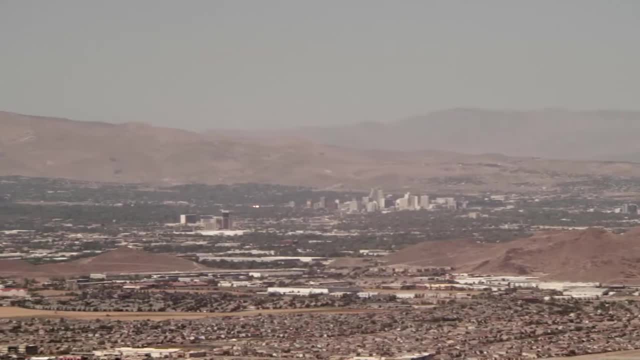 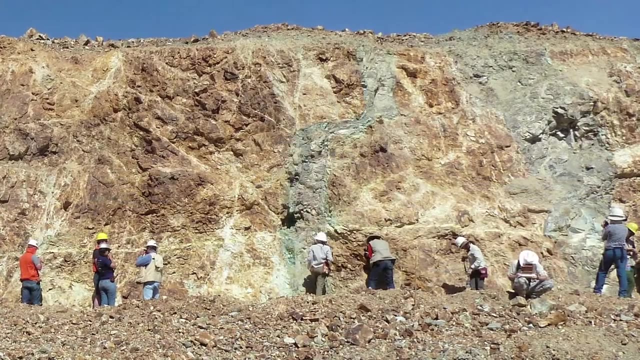 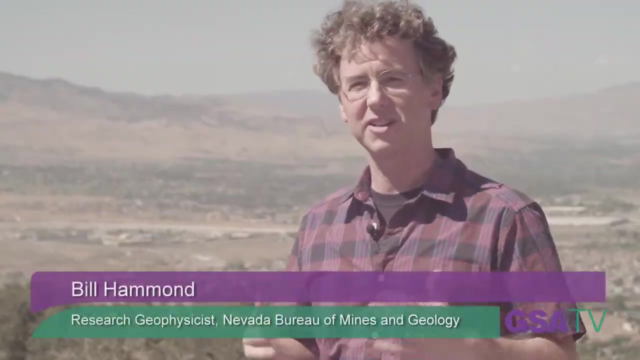 in the Reno Carson City urban corridor. One of the most important activities of the Nevada Bureau of Mines and Geology is studies on individual faults that pose hazards to the state of Nevada. One of the things that makes Nevada special- a special place to study earthquakes, tectonics- is that Nevada 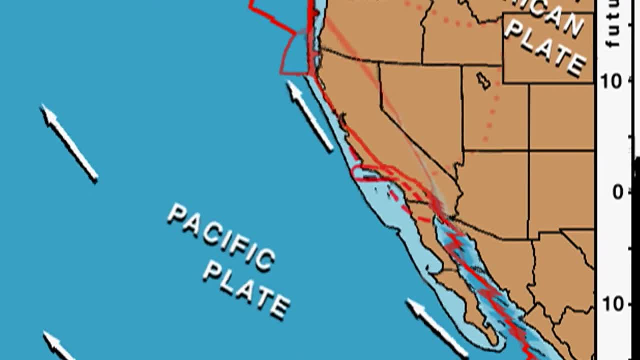 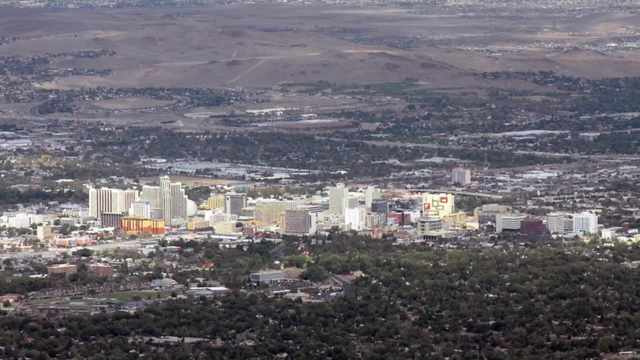 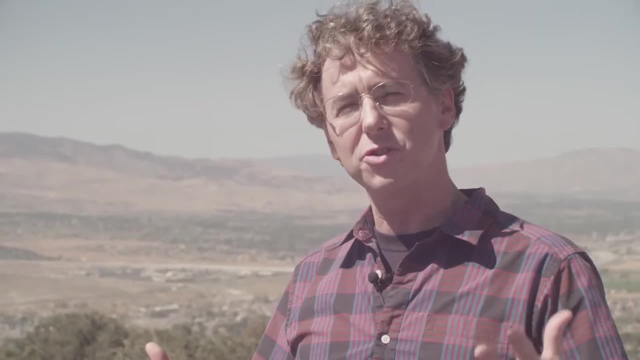 is constantly undergoing tectonic strain. Nevada is a state that's constantly growing because of active tectonic processes. Reno Nevada sits in a basin that's been formed through active tectonic processes. With research that we do at the Nevada Bureau of Mines and Geology, we can measure the active 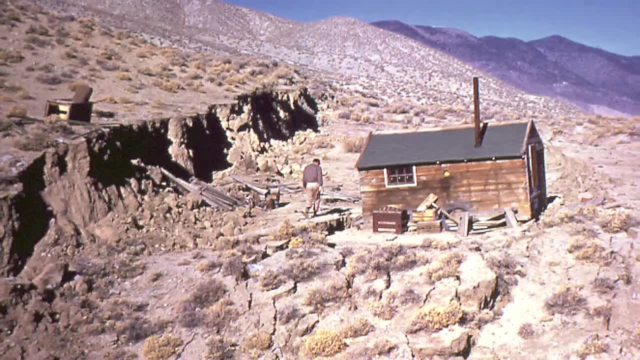 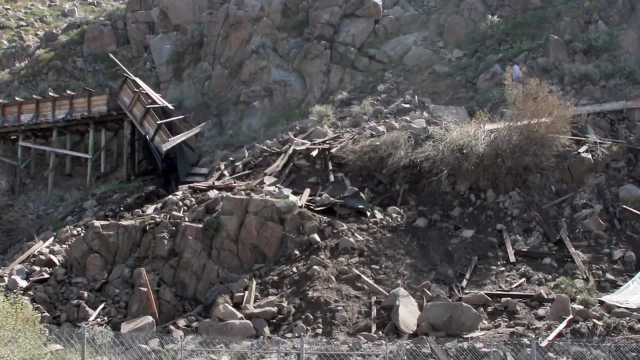 tectonic deformation of this basin and others. We know about faults that exist. Earthquakes around Reno Nevada, to the east and to the west that are experiencing slip over time. Earthquakes pose a significant hazard for the residents of Nevada. Nevada is actually. 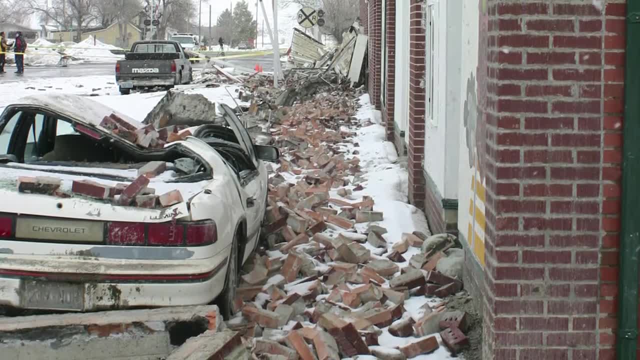 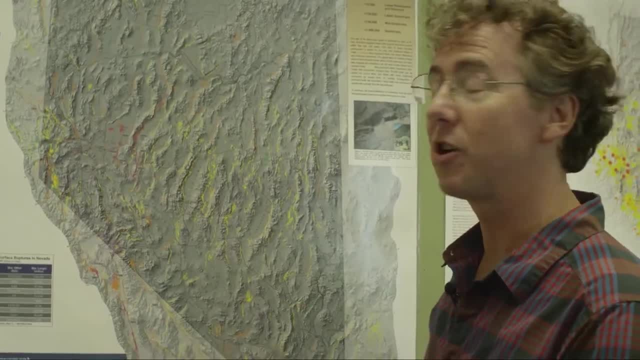 the third most seismically active state after California and Alaska. One of the studies that have been recently performed by the Nevada Bureau of Mines and Geology is on the Genoa Fault, which bounds the west side of the Carson Valley. This fault can slip between three and five meters in individual earthquakes, and those earthquakes 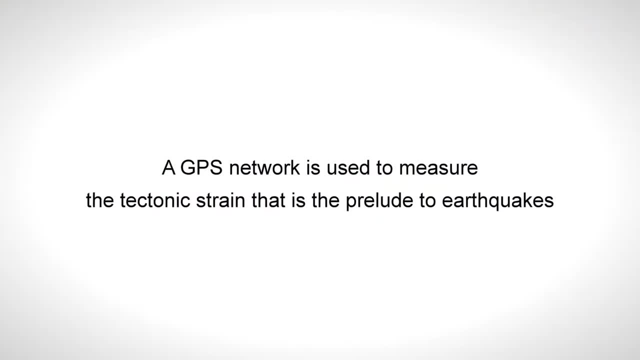 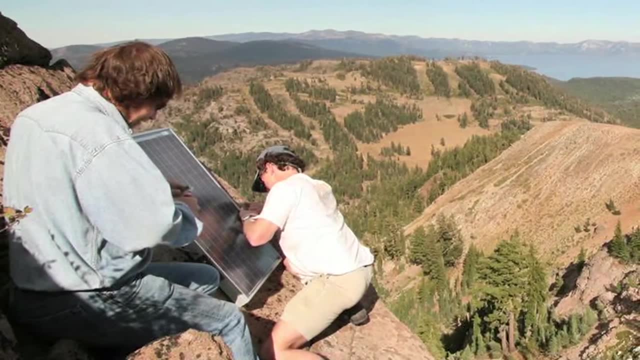 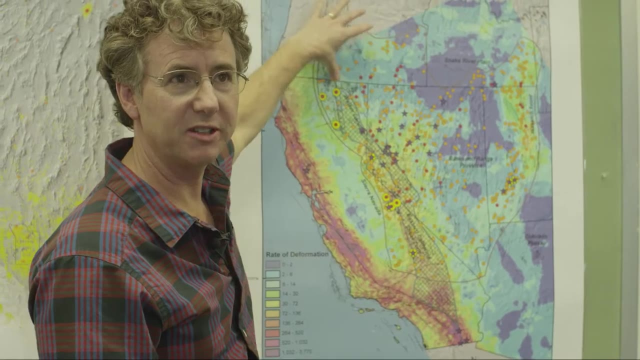 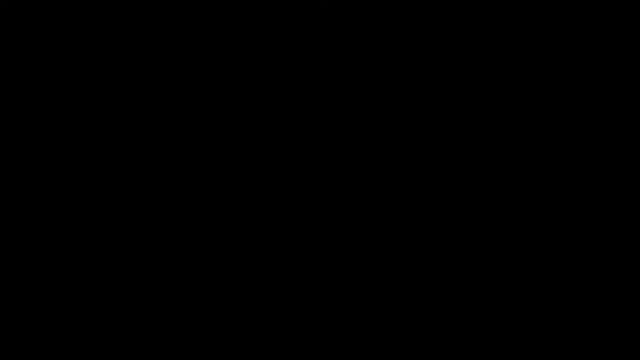 occur every two to three thousand years. czyndor tatsächlich. And this is where we innovation is happening. This is where we collect the geodetic measurements in order to produce maps that you can see. Nevada has vast geothermal resources- more than any other state- And the detailed research. at the Bureau. let's you realize🏦jbrqaesimov. something we mask that's not worth a grand sum and much morequer. This is in order, to feel, to reduce the amount of terrorists leaving and gathering their artificial land regeneras, load treatment as low as temporary pressure in the atom of what's, however, not possible During the visit to Arizona. they're observing us and that's also important. Now let's explain the details of maps and the maps. So this has gone to the World: Gechied and our 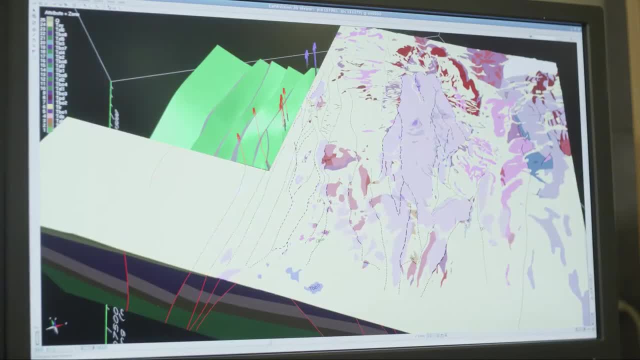 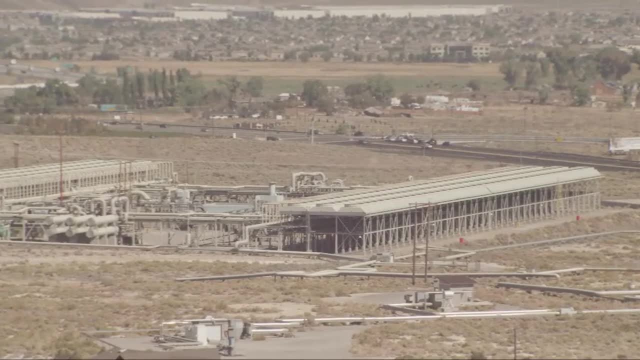 area of DRRLEвер. Nevada has vast geothermal resources, more than any other state. The detailed research at the Bureau has led the discovery of about a dozen new geothermal systems and also to enhancement of several existing geothermal systems. We estimate that probably about three quarters of the resources are blind or hidden. 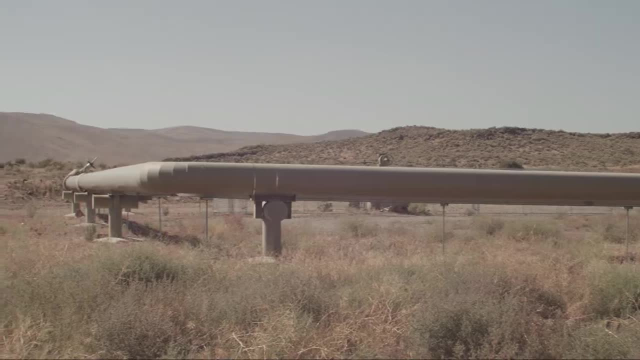 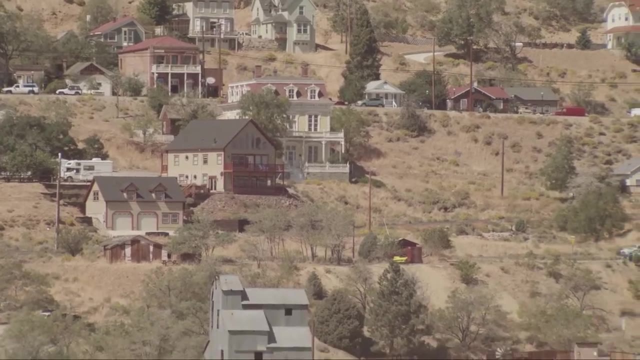 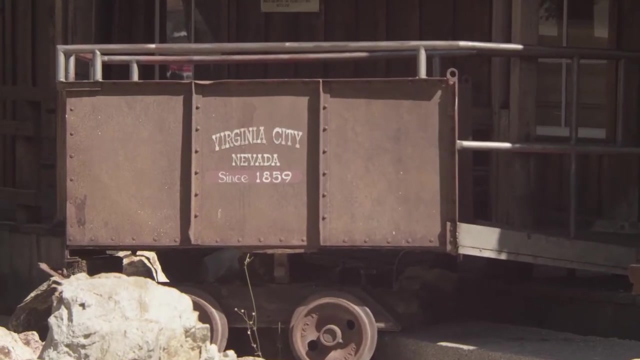 And so one day, if those resources are developed, Nevada could be an exporter of energy to other parts of the country. Behind me is Virginia City, where mining began in Nevada in 1859, with the discovery of the fabulously rich Comstock Loeb. 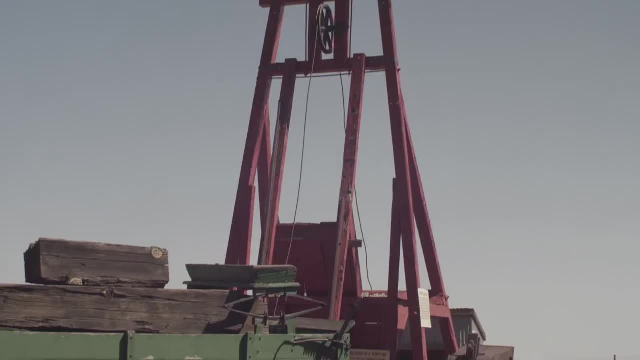 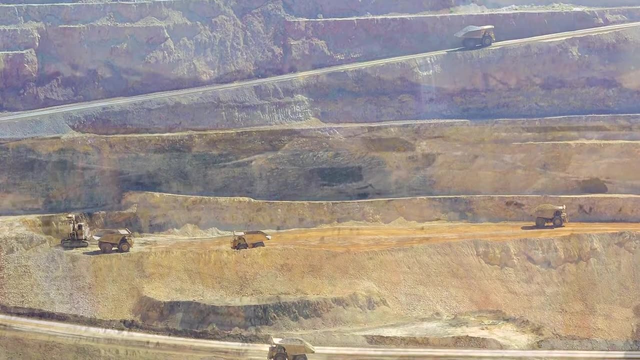 Nevada is the leading producer of gold in the United States, producing 5.5 million ounces of gold, third in the world behind China and Australia. Now, the Nevada Bureau of Mines and Geology plays a critical role in sustaining Nevada's vibrant mining industry. 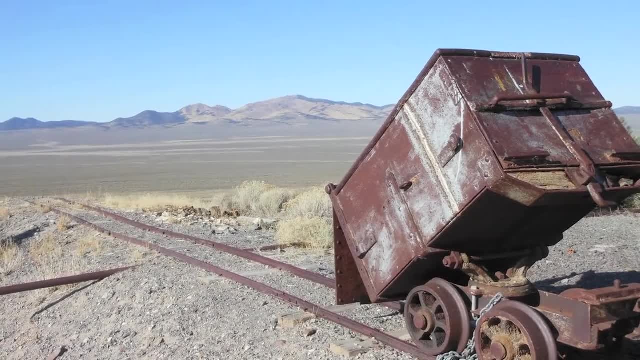 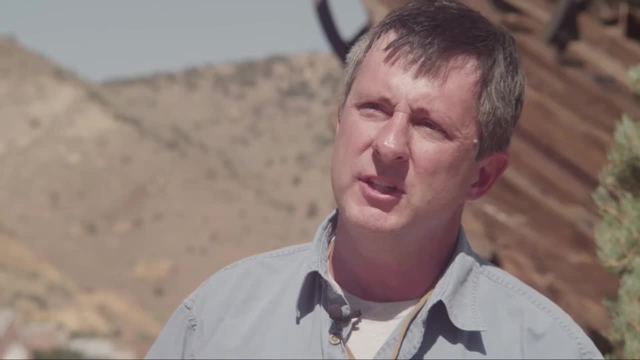 That industry has an $8 billion impact on Nevada and employs 10,000 people at an average salary of over $80,000 a year. The research that the Nevada Bureau of Mines and Geology does on ore deposits addresses the two critical questions that gold explorers face. 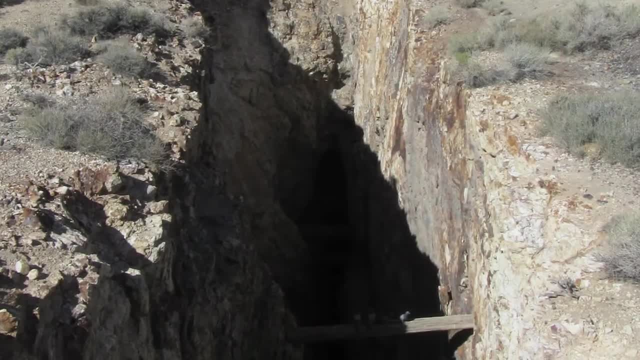 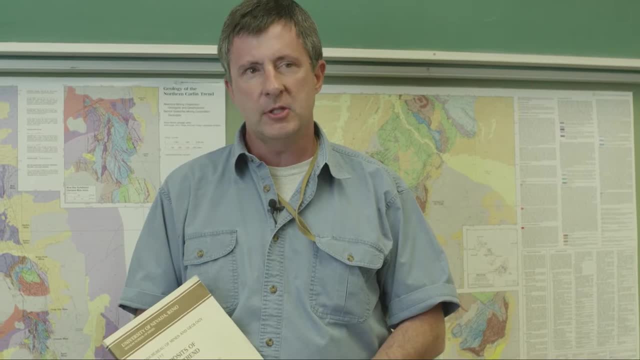 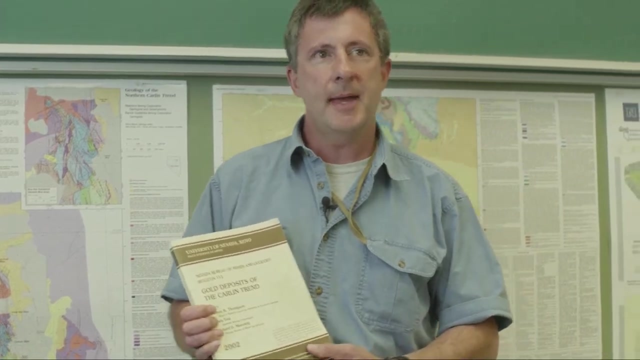 First, where do you look? And secondly, once you're in the right place, how do you vector in to the actual ore body that they can mine? Another way Nevada Bureau of Mines and Geology helps companies find gold deposits is through our reports and maps. 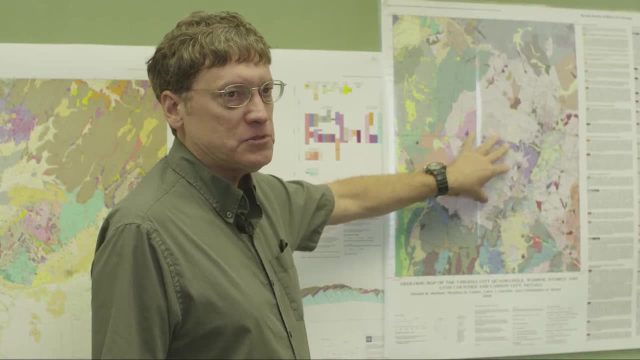 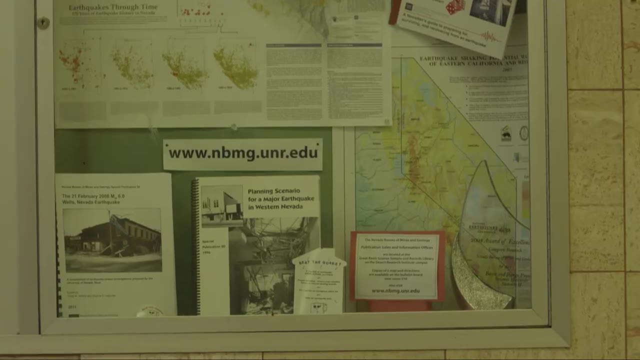 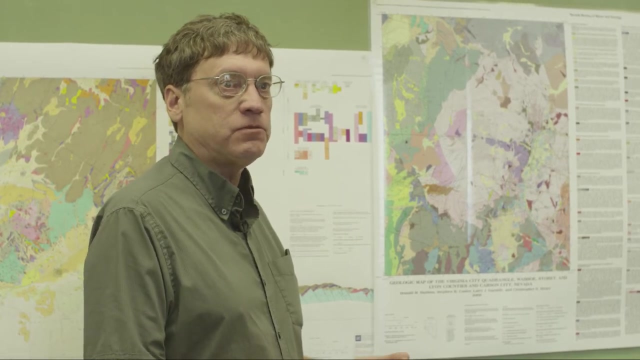 A geologic map shows the distribution of rock types And faults, and some of these are earthquake faults, And that distribution of rock types and faults helps us understand or be able to assess things like mineral resources, geothermal resources, natural hazards like earthquake faults, flood. 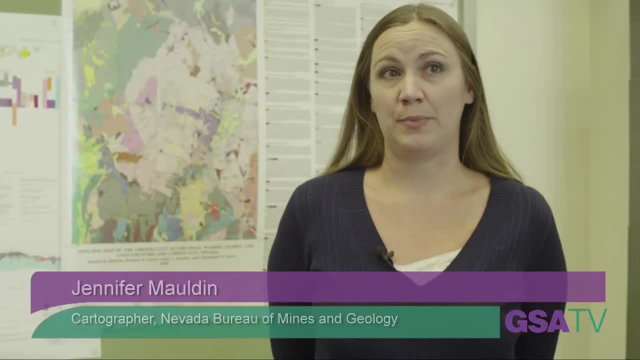 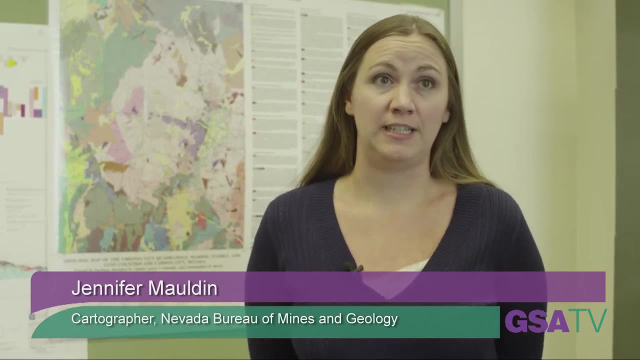 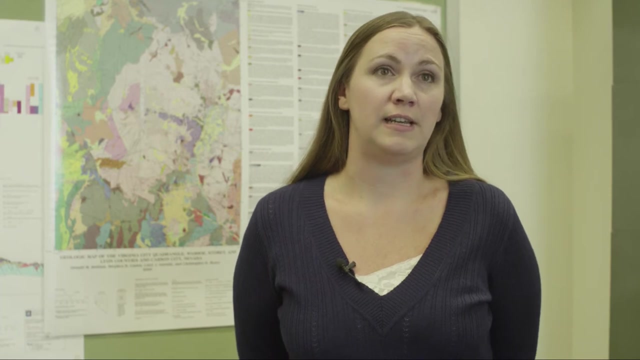 hazards and that type of thing. Our cartography and GIS department is a specialty group within MBMG that produces maps and publications for our faculty students and staff within MBMG but also around campus. It's a resource that other departments can come to. 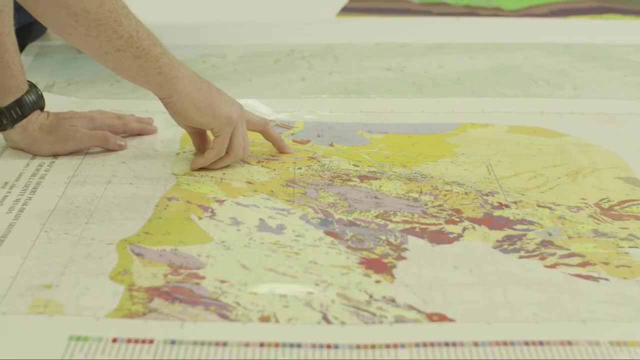 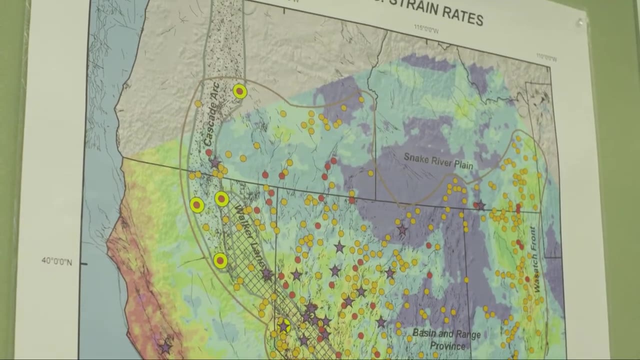 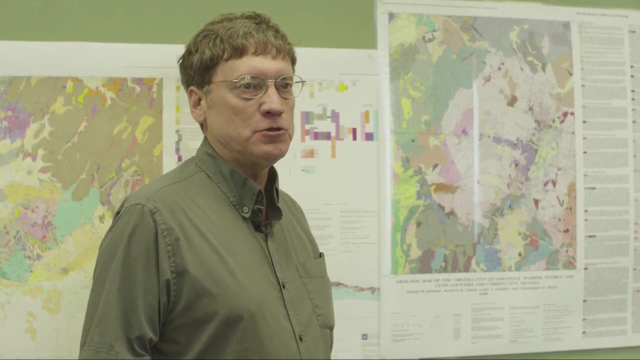 Not only does our department support campus faculty staff and students, we also support other agencies around the state and also federal agencies. With only 20% of the state mapped at a useful scale, an important part of the Bureau's future is to continue that mapping- mapping the remaining 80% of the state. it would be very important. 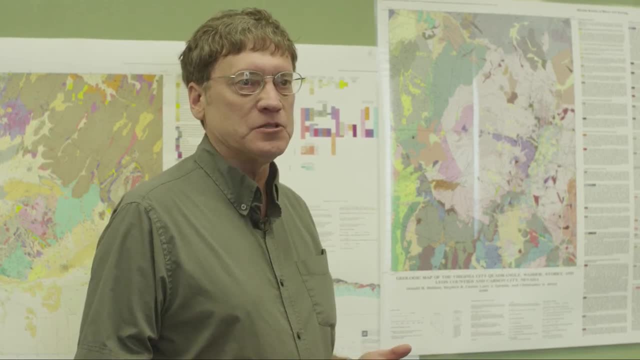 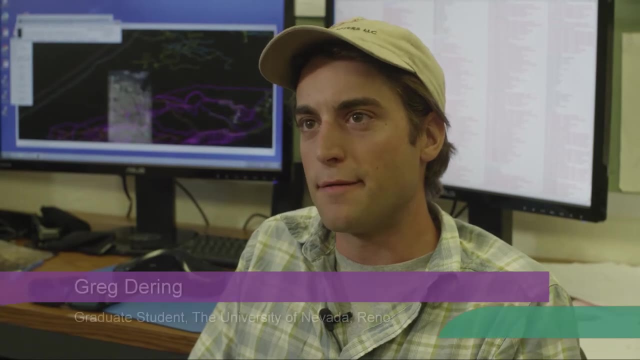 for understanding geosciences, Thank you. Pharma Resources, Mineral Deposits, Natural Hazards like Earthquakes: Nevada Bureau of Mines and Geology involves students in this research. The Bureau was definitely a factor in me choosing the University of Nevada at Reno. 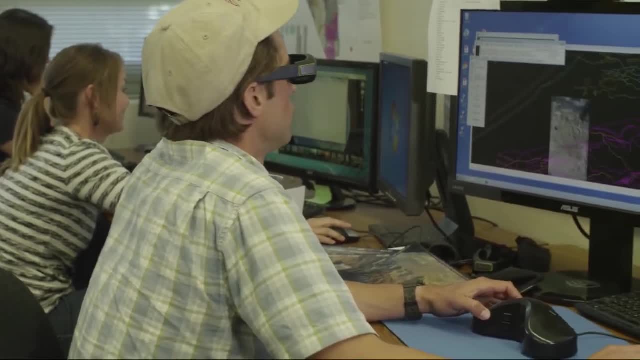 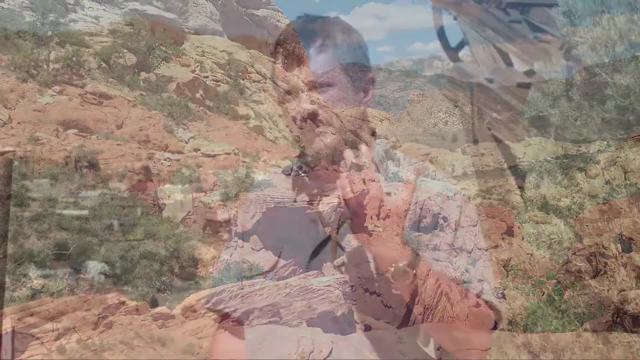 Well, I feel really prepared to go out in to the work world at this point because I've been working around a lot of professional geologists for the past couple years. The baseline data on previous maps, geochemical data, libraries of old samples- plays a critical 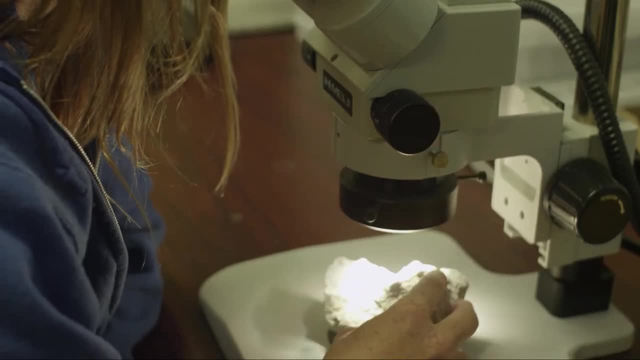 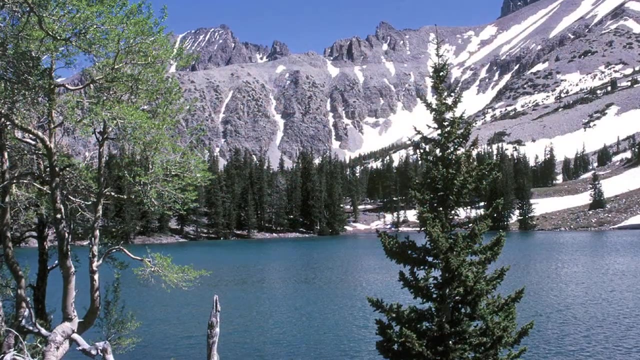 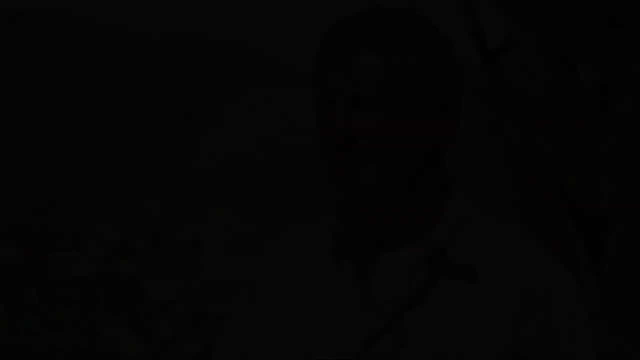 role in the exploration process. The research at the Nevada Bureau of Mines and Geology is crucial in a state like Nevada, because 87% of Nevada's land is federally managed, So that research is very important in making good decisions on the use of that land. 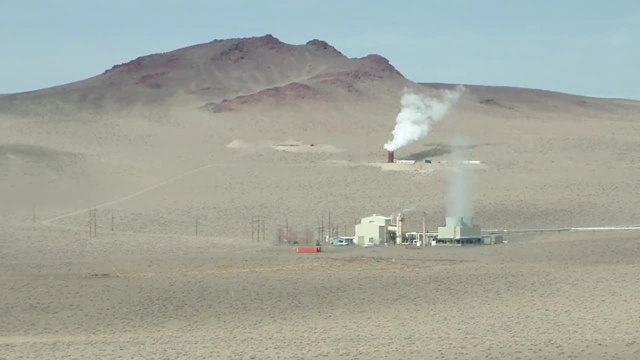 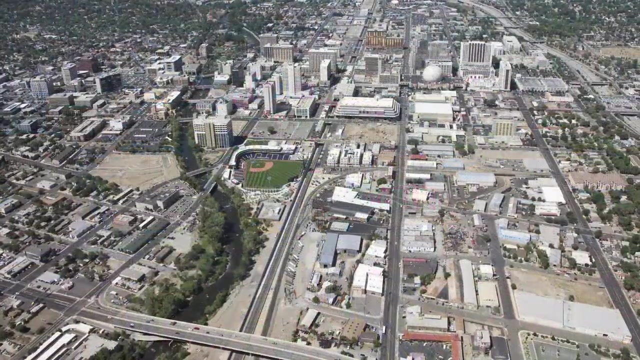 The research of the Nevada Bureau of Mines and Geology is critical for developing energy resources in the future and mitigating natural hazards such as floods and earthquakes in Nevada's growing cities. 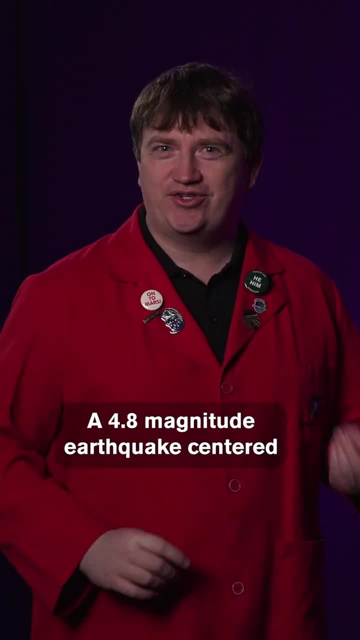 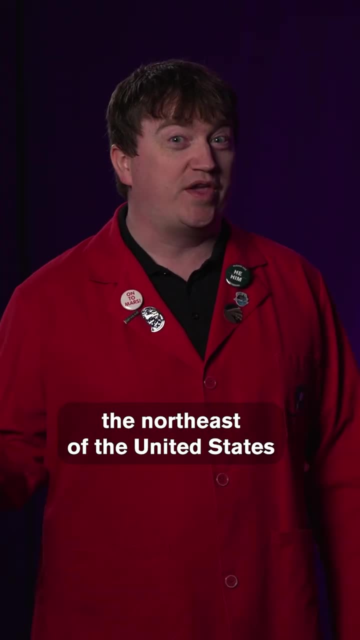 Did you feel that earthquake? A 4.8 magnitude earthquake centered in New Jersey shook buildings in New York City and was felt as far away as Boston? Typically, we don't associate the northeast of the United States with earthquakes. We think more in terms of California or around. 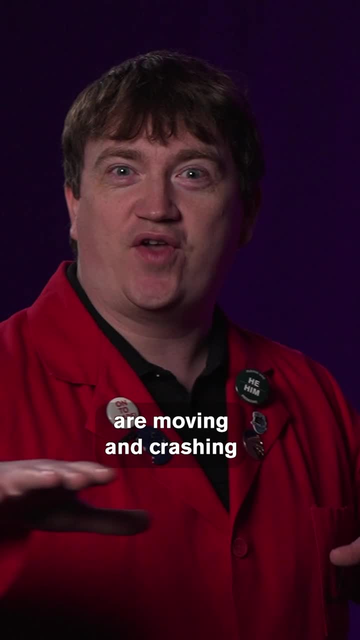 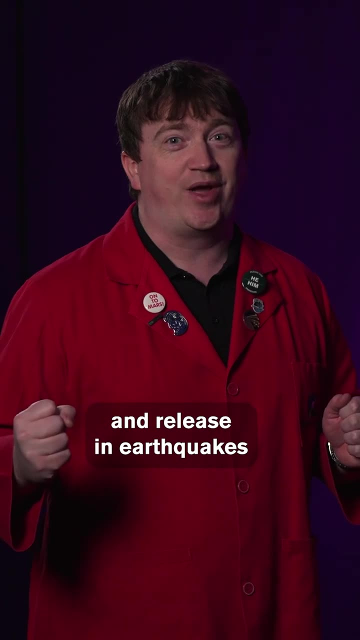 the edge of the Pacific Ocean. Those are places where the Earth's tectonic plates are moving and crashing into each other or pulling apart. Some of that activity can build up stress under the ground and release in earthquakes In the middle of those tectonic plates, like 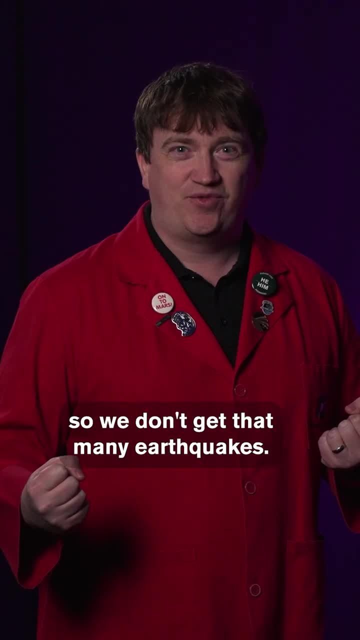 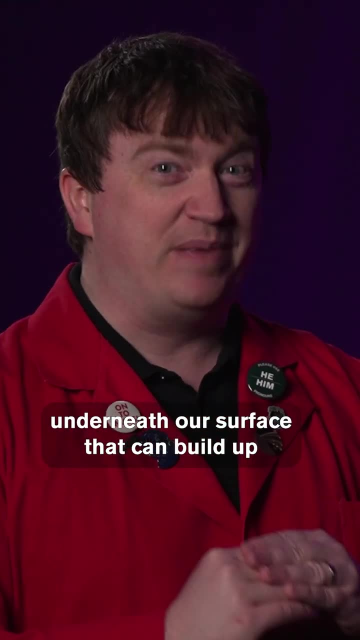 in the northeast. we're far away from all of that activity, so we don't get that many earthquakes, although there are still some imperfections and fractures underneath our surface that can build up a little extra stress and release it in the form of smaller, less. 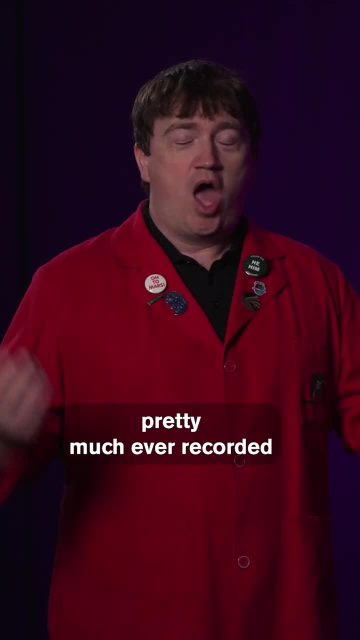 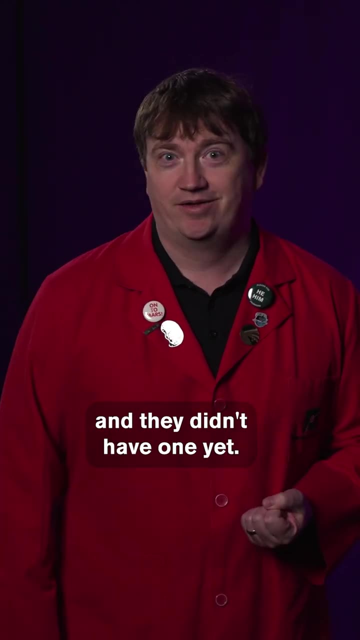 frequent earthquakes. This one in New York City was the most powerful one pretty much ever recorded, because the last time there was a significant one in New York City, the seismometer had barely been invented and they didn't have one yet. Have you felt an earthquake?